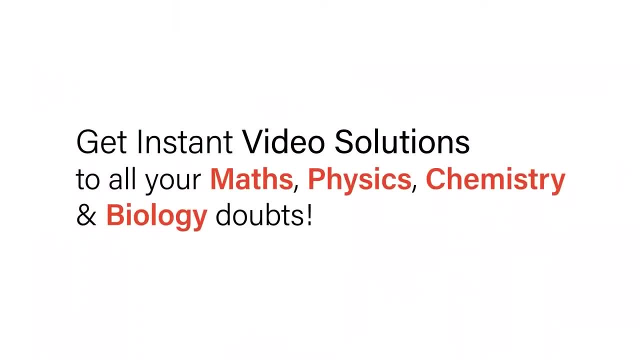 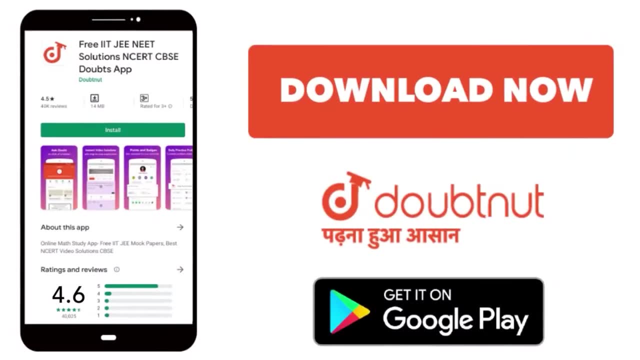 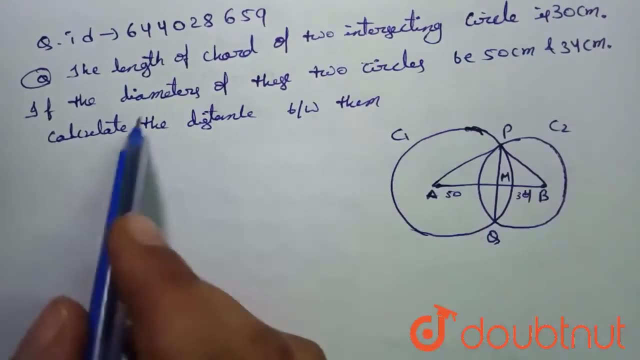 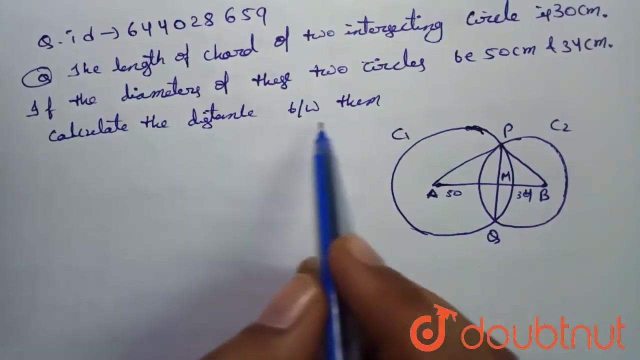 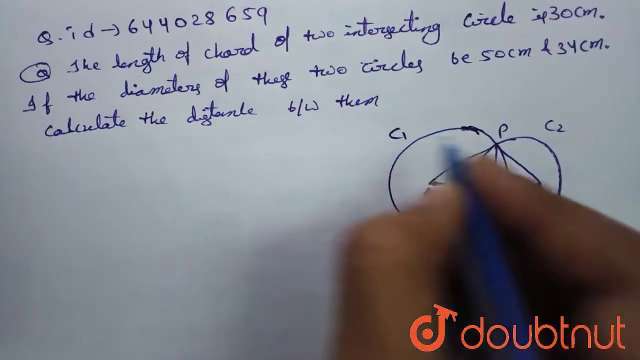 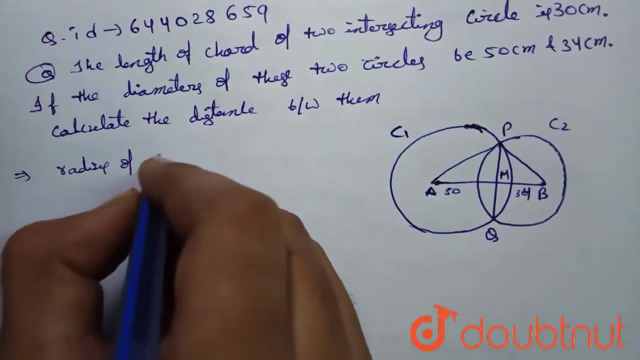 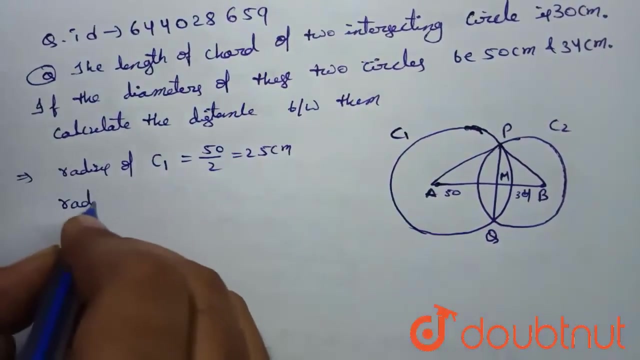 With Doubtnit, get instant video solutions to all your Maths, Physics, Chemistry and Biology doubts. Just click the image of the question, crop the question and get instant video solution. Download Doubtnit app today. We consider this as circle 1 and this as circle 2.. This implies radius of C1- circle 1- is equal to 50 by 2, which is equal to 25 cm, and radius of C2- that is, circle 2- is 34 divided by 2 is equal to 17 cm. 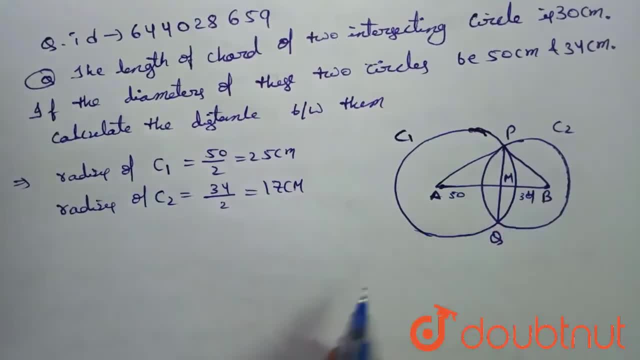 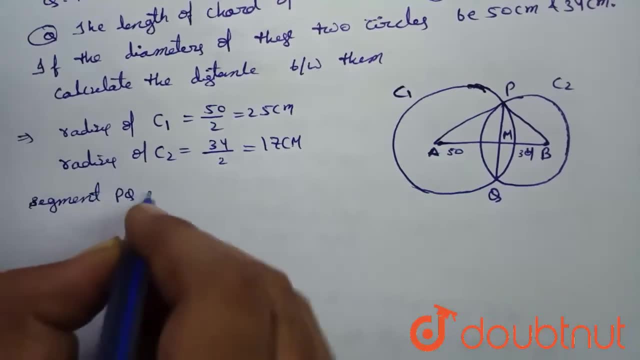 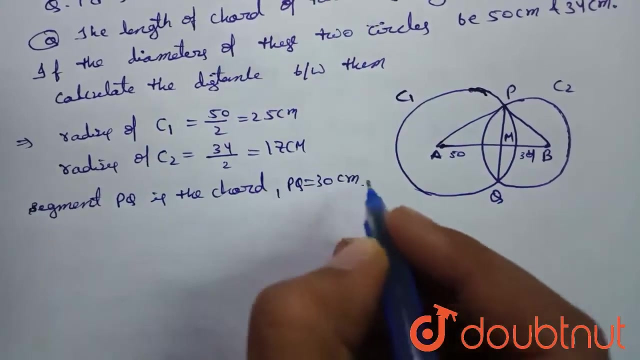 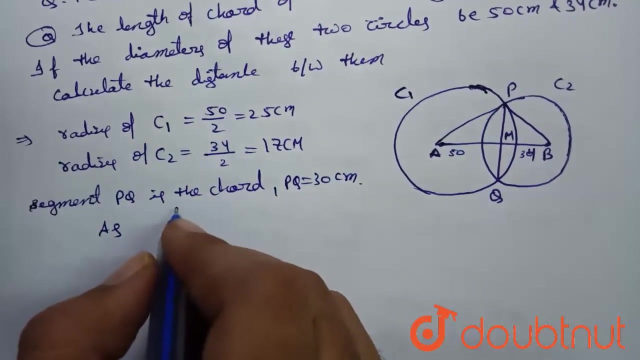 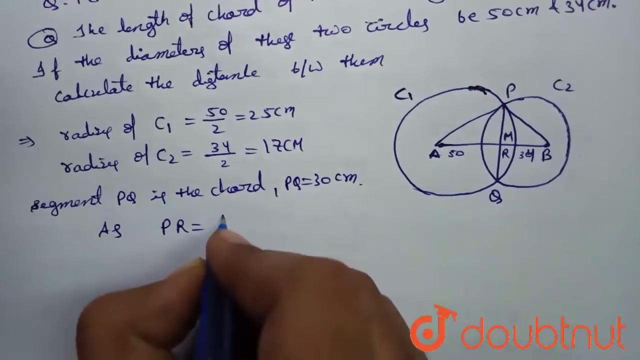 The segment PQ is called common chord. PQ is equal to 13 cm, as given. as PR is equal to PQ divided by 2, which is equal to 15 cm. PR is equal to PQ divided by 2, which is equal to 15 cm. 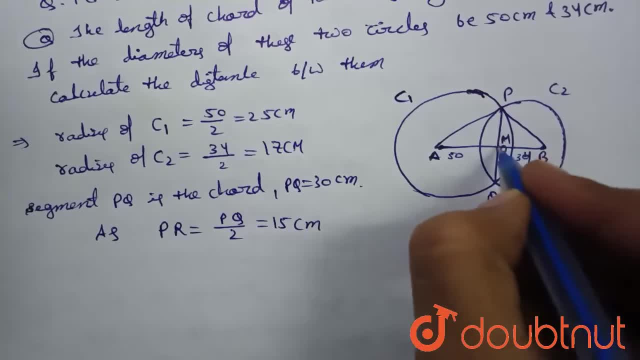 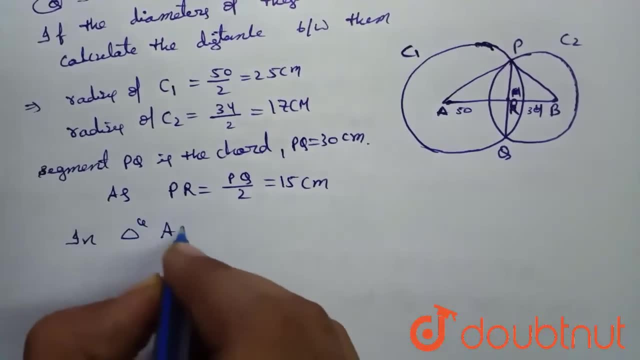 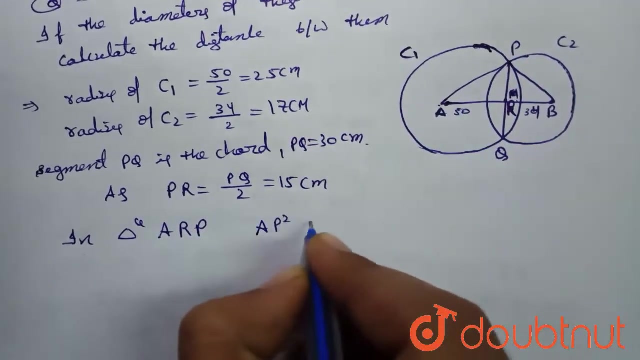 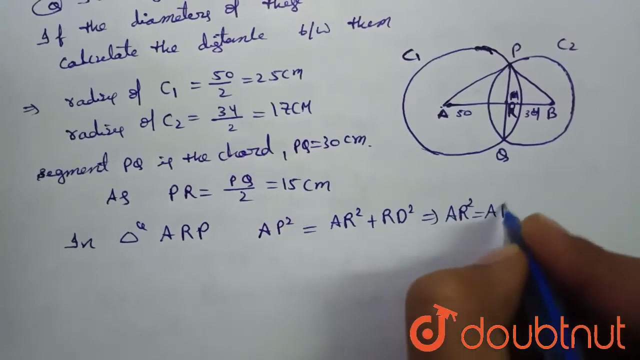 PR is equal to PQ divided by 2, which is equal to 15 cm divided by 2. this is r. this is the midpoint in triangle arp- arp. using the pythagoras theorem, ap square is equal to ar square plus rd square. this implies ar square is equal to ap square. 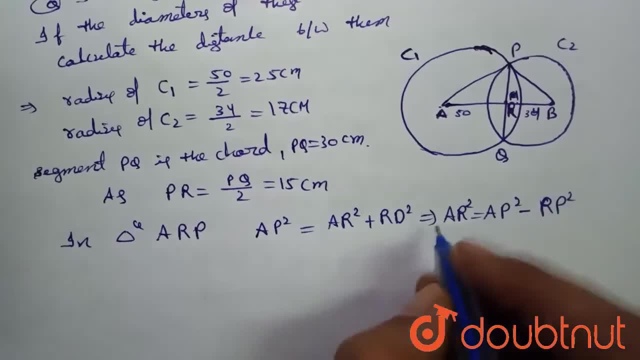 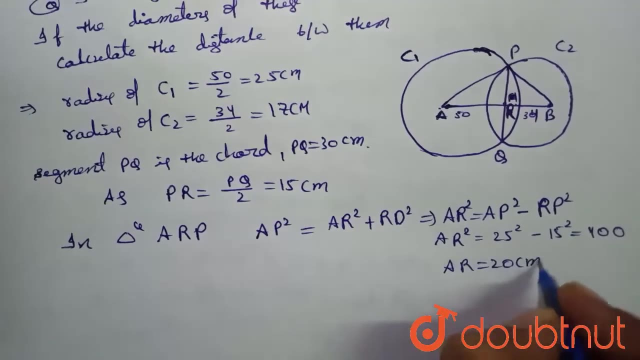 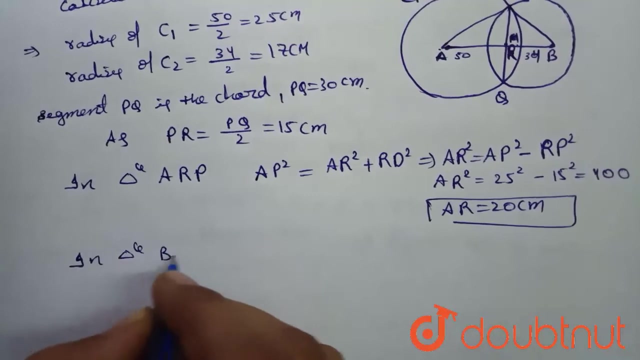 minus rp square, ar square is equal to 25 square minus 15 square, which is equal to 625. minus 225, which is equal to 400, ar is equal to 20 centimeter. and now, in triangle, b r p using the pythagoras theorem, bp. 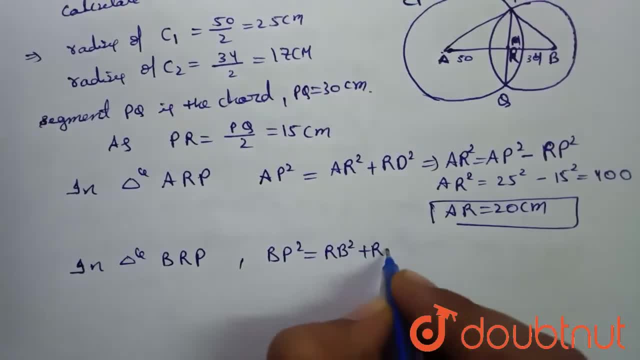 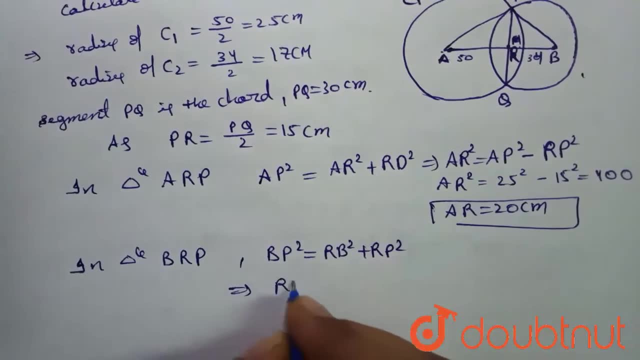 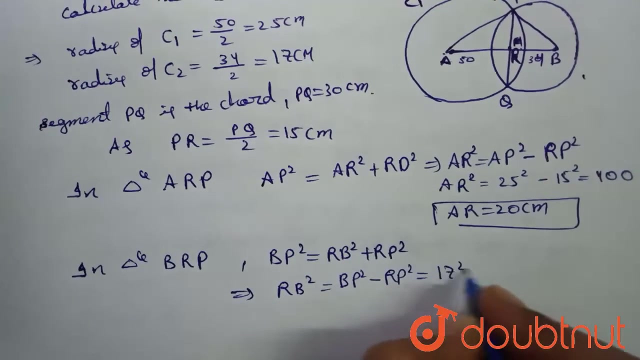 square is equal to 25 square minus 15 square, which is equal to 625 minus 225, which is equal to rb square plus rp square. bp square is equal to rb square plus rp square. this implies rb square is equal to bp square minus rp square, which is equal to 17 square minus 15 square.